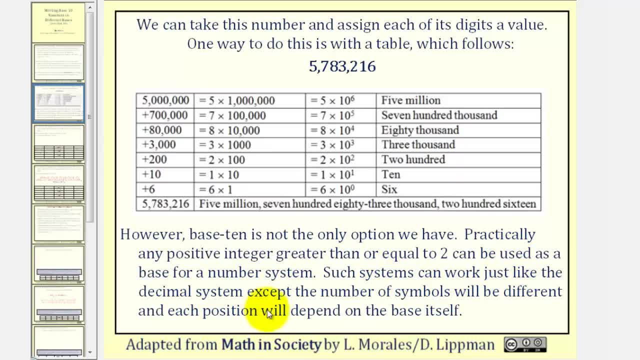 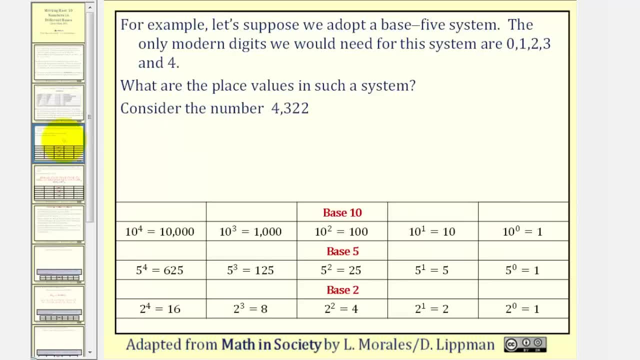 system. Such systems can work just like the decimal system, except the number of symbols will be different and its position will depend on the base itself. For example, let's suppose we adopt a base five system. The only modern digits we would need for this system are zero. 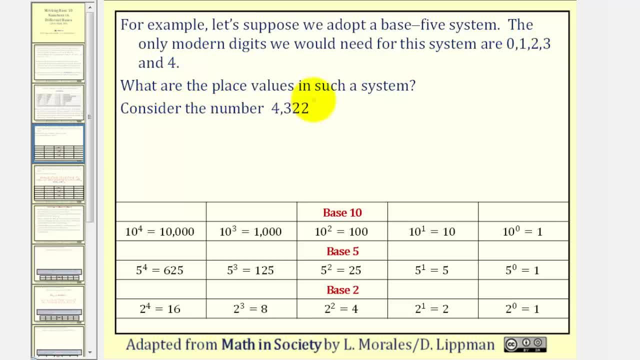 one, two, three and four. So to determine the place values in such a system, we would take the base five, start with five to the zero, which would give us the ones place value, and then start increasing the exponent by one. Five to the first would give us the fives. 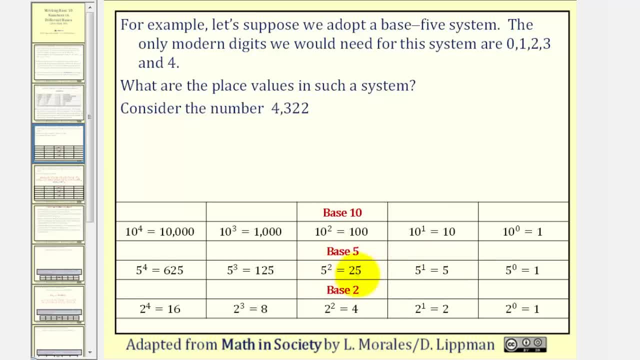 place value. five to the second would give us the twenty fives place value. five to the third would give us the one hundred twenty fives place value, and so on. So by knowing the base we can determine the value of each place value. As an example, 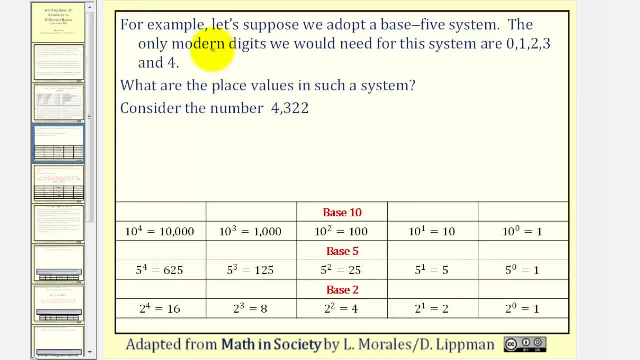 four thousand three hundred twenty two. we know in base ten which we could indicate with a small ten. here The four means four, one thousands, the three means three, one hundreds, the two here means two tens and this two means two ones. But if we change this to base, 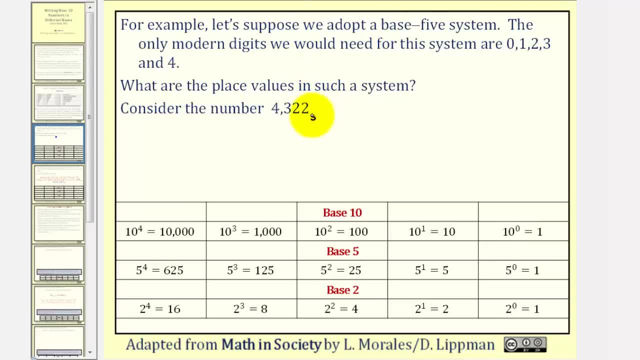 five. now. the four is going to be the one hundred and the one hundred is going to be. three represents four, five to the thirds, or four, one hundred twenty fives. The three indicates three, five to the seconds, or twenty fives. This two here means two, five to the. 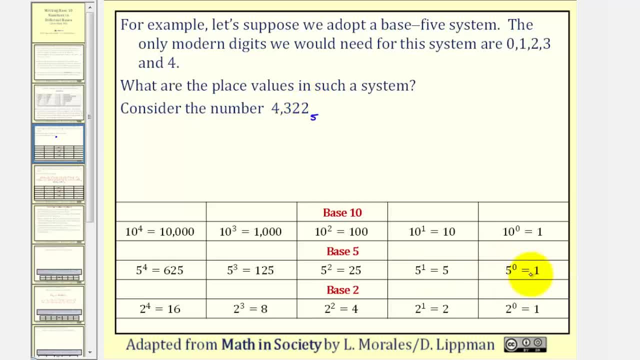 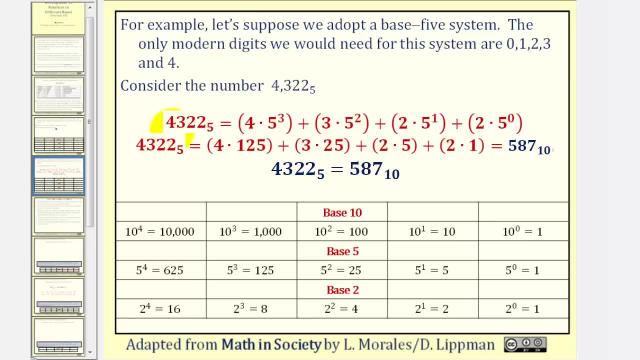 first or two fives, and this two means two ones. So if we wanted to determine the value of this number in base ten, we could do so by multiplying the digit by its place value, as we see here. So if we simplify, on the right notice how we get five. 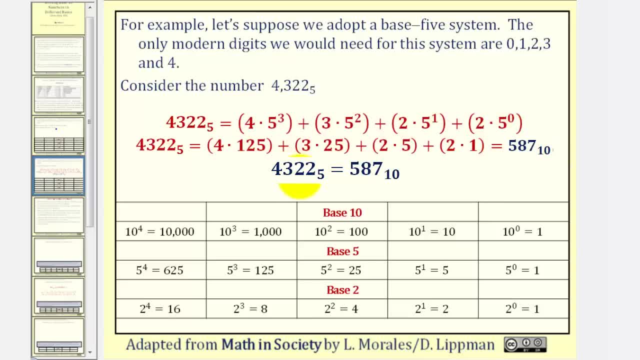 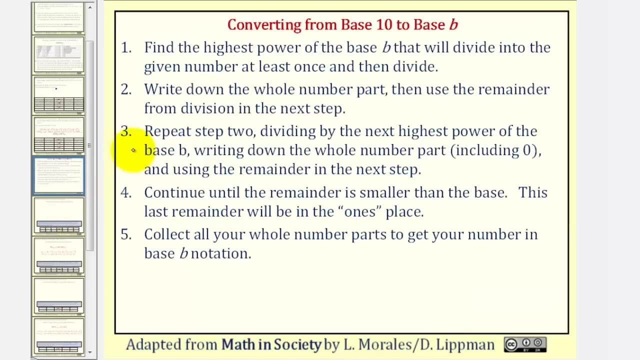 hundred eighty seven in base ten. So we can say that four, three, two, two in base five is equal to five hundred eighty seven in base ten. But in this lesson we'll focus on how to convert a number in base ten to a different base And we're going to use what's called 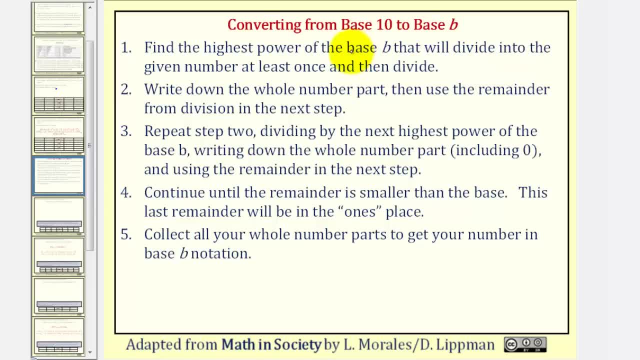 the remainder method. In another video we'll take a look at how we can use decimals to do these conversions using a calculator. So for the remainder method, to convert base ten to base b, number one, we'll find the highest power of the base. 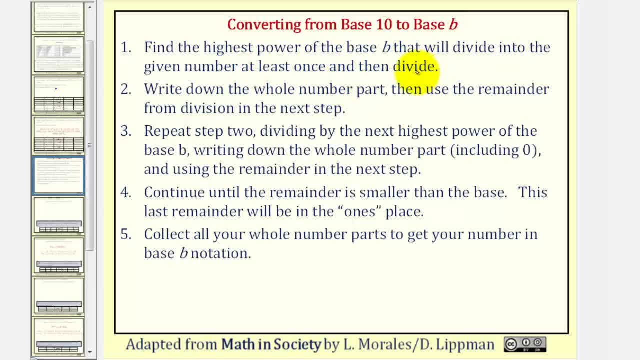 that we'll divide into the given number at least once and then divide. Step two: we'll write down the whole number part, then use the remainder from the division in the next step, Step three. we'll repeat step two, dividing by the next highest power of the base b. 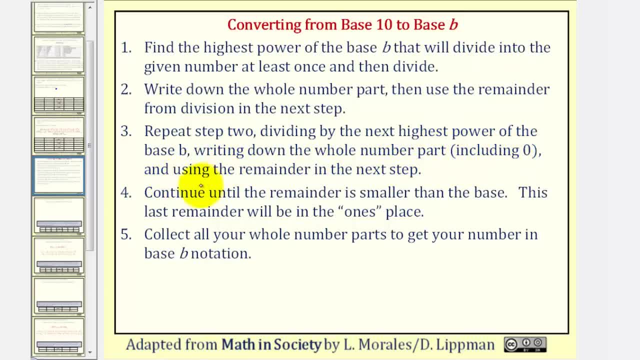 writing down the whole number part, including zero, and using the remainder in the next step. Step four: continue until the remainder is smaller than the base. this last remainder will be the one's place. Step five: collect all your whole number parts to get the number in base b notation. 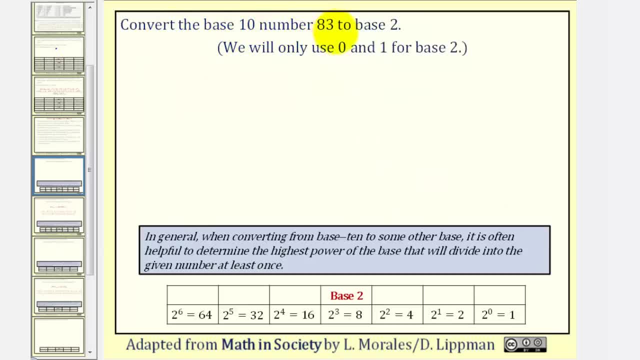 So let's take a look at two examples. We want to convert the base ten, number eighty three, to base two. To begin, I'd like to write out the place values in base two. So we'll start with two to the zero power, which is equal to one, and then we'll increase the exponent by one to four and then divide. 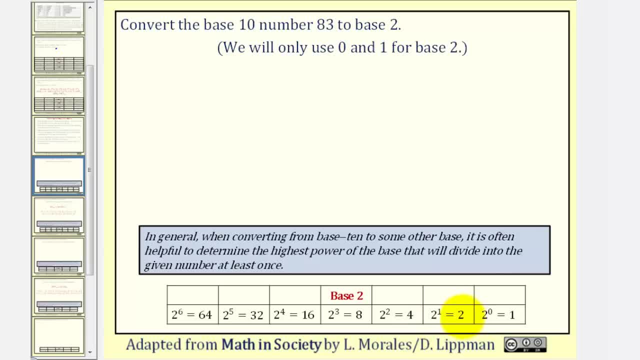 to find several more place values. So two to the first gives us two, two to the second four, two to the third eight, two to the fourth 16, and so on. This indicates the place values for base two. 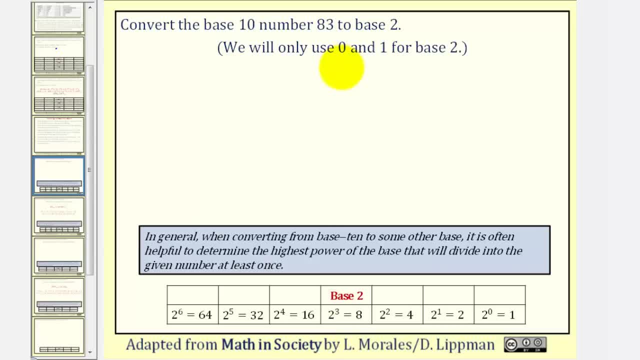 And now we're looking for the highest power of two that we'll divide into the given number, 83, at least once, Notice that that would be two to the sixth, or 64,, because two to the seventh would be too large. 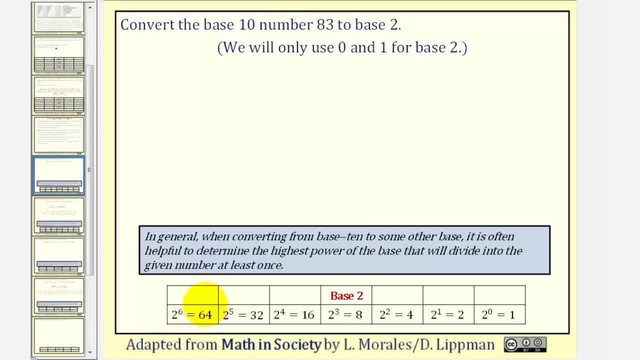 So, because we know that two to the sixth is the highest power of two, that divides at least once into 83, we know our number in base two is going to have one, two, three, four, five, six, seven digits, So let's go ahead and leave room for all seven digits. 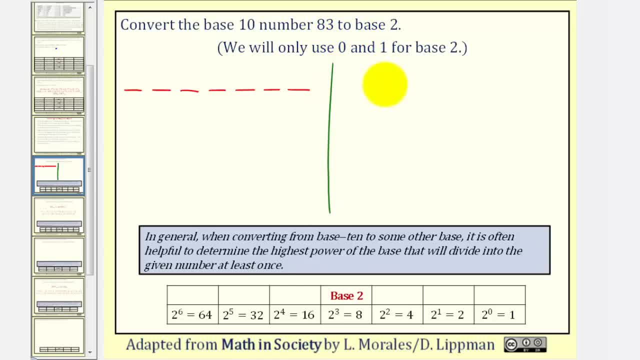 And now we'll start dividing. We'll divide 83 by 64.. 64 divides once into 83.. One times 64 is 64.. Notice, here we have a remainder of 19.. The whole number, part of our quotient, in this case one. 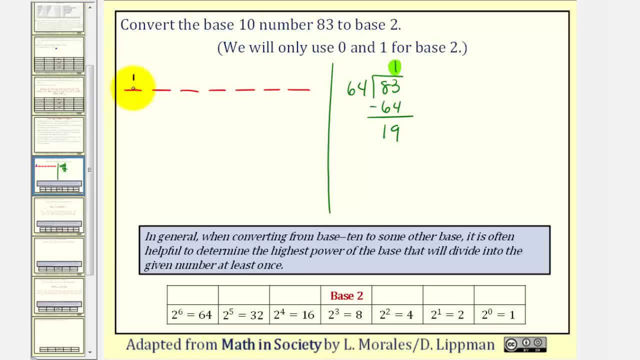 gives us the digit in the two to the sixth place value, which is here. Now we repeat the process with 19.. We're looking for the highest power of two that divides at least once into 19.. Notice, two to the fifth is too large. 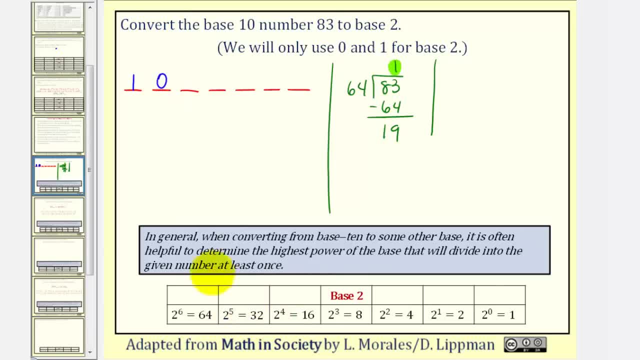 which means we'll have a zero and the two to the fifth, which is zero, and the two to the fifth place value, And then we go to two to the fourth, which is 16.. 16, we'll divide it in 19, at least once. 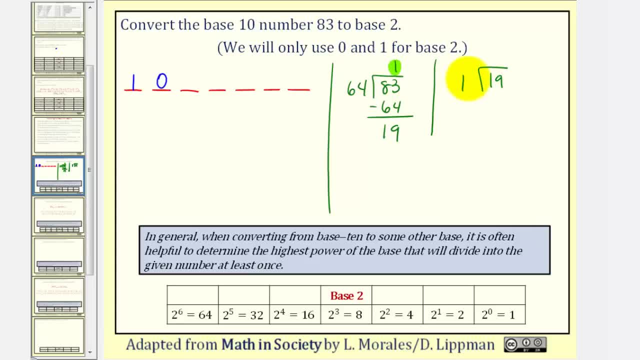 So now we'll take 19 and divide by 16. Goes in one time and now we have a remainder of three. So the whole number one gives us the digit in the two to the fourth place value, which is here, And we repeat the process with three. 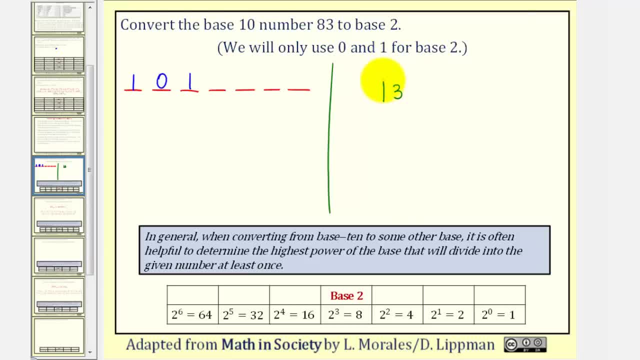 We're going to find the highest power of two that will divide at least once into three. Well, two to the third, or eight, is too large, which means we'll have a zero in the two to the third place value, which is here. 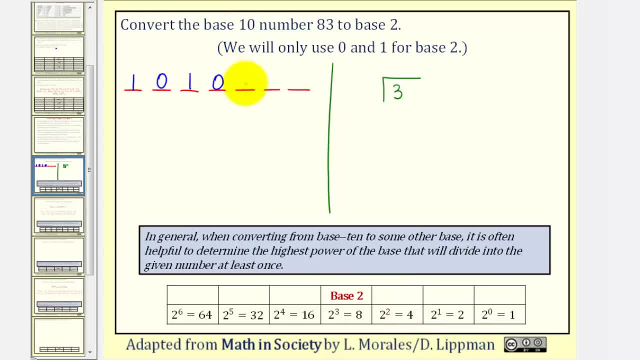 Two to the second or four is also too large, so we'll have another zero in this place value, which brings us to two to the first or two. So three divided by two is equal to one. One times two, of course, is two. 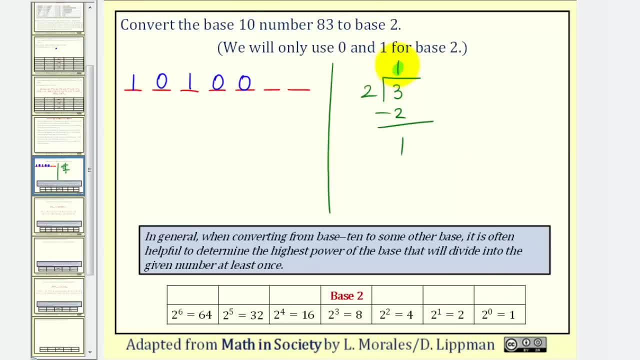 We subtract, the remainder is one. This one goes into the two to the first or the two place value, which is here. This remainder is less than the base, which gives us the digit in the one's place value, which would be here. 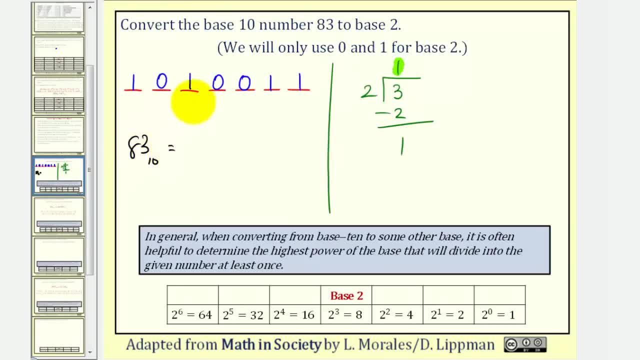 So what we found is: 83 in base 10 is equal to 1010011 in base two. Of course, if we want to check this, we can go in the reverse order, which I've already done to save some time. Notice how this one is in two to the sixth place value. 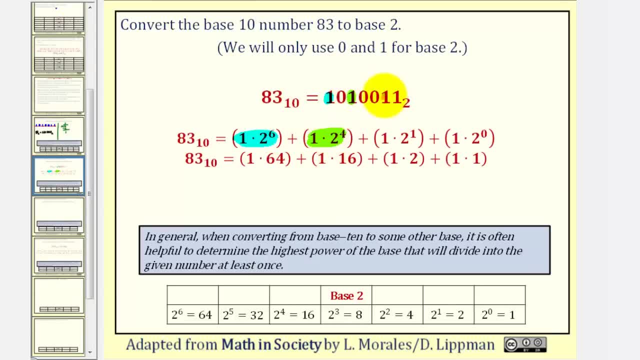 This one here is in the two to the fourth place value, This one is in the two to the first place value And, finally, this one is in the two to the zero, or one's place value If we find the sum of these products. 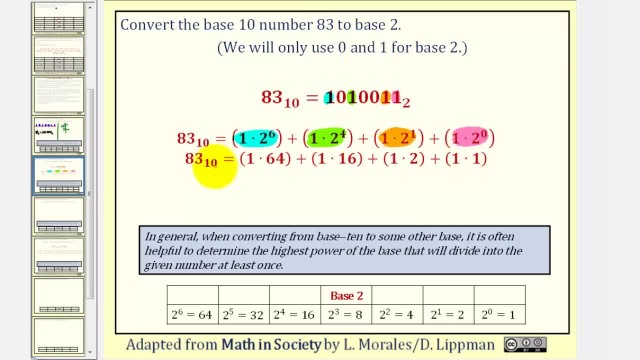 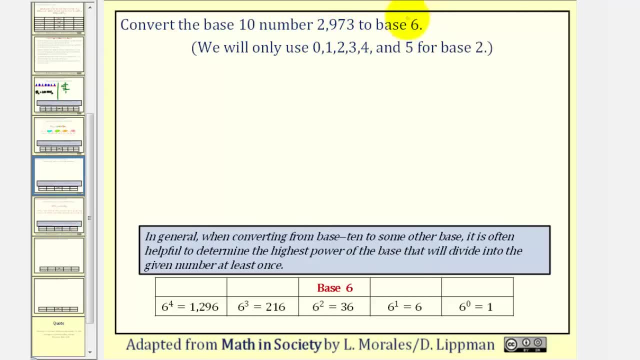 it does give us 83 in base 10.. Let's take a look at one more example. We want to convert the base 10 number 2973 to base six. so again, we first want to find the place values by starting with six to the zero. 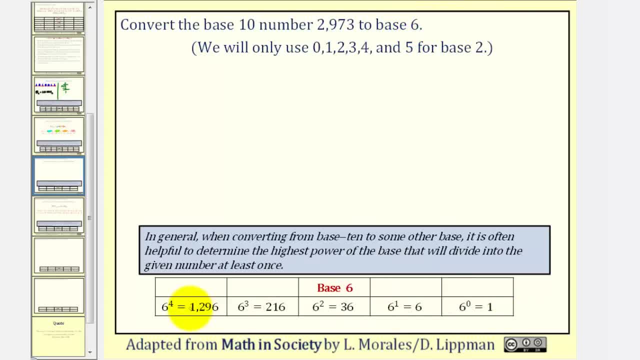 increasing the x one by one to find several place values to the left, which we see here: Six to the first, six to the second, six to the third, six to the fourth and so on. I just noticed this should say we only use zero through five for base six, not base two. 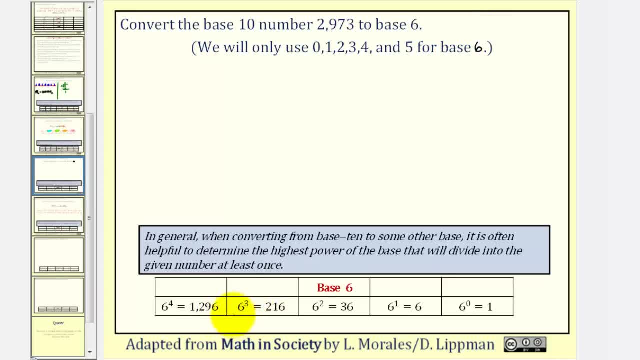 Now we begin by determining the highest power of six. that we'll divide, at least once, into 2973, by six to the fourth, because six to the fifth would be too large, Which means our number in base six is going to have one, two, three, four, five digits. 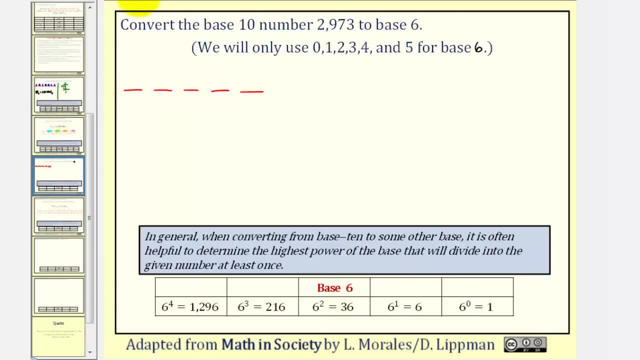 So one, two, three, four, five. Now we begin by dividing 2,973 by six to the fourth, or 1,296.. This divides in two times. so two times our divisor is 2,592, and this difference of the remainder is 381.. 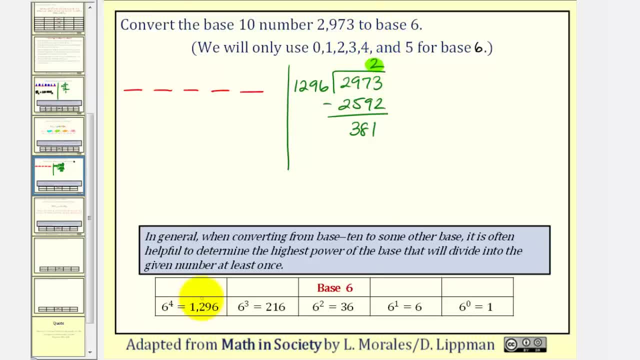 So the whole number of two gives us the digit in the six to the fourth place value which is here. Now we repeat the process using the remainder of 381.. We want to find the highest power of six. that'll divide at least once into 381.. 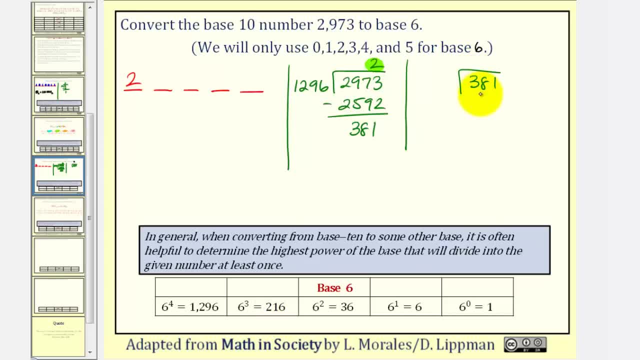 And notice how 216 would divide at least once into 381. So now we'll divide by 216 to find our next digit. 216 goes once into 381.. We subtract the remainder as 165.. So one is our next digit. 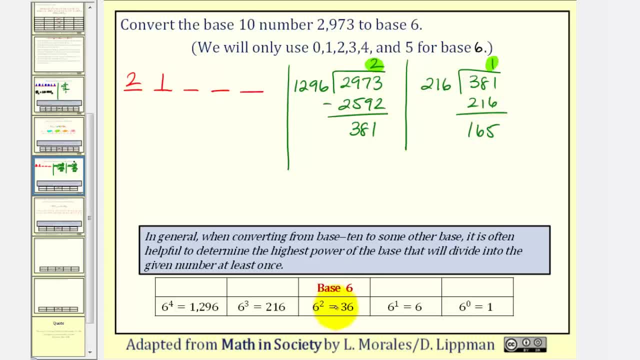 Now we repeat again: We're going to determine the highest power of six. that would divide into 165 at least once. And notice how six- The second of 36- we'll divide at least once into 165.. So we take 165 and divide by 36.. 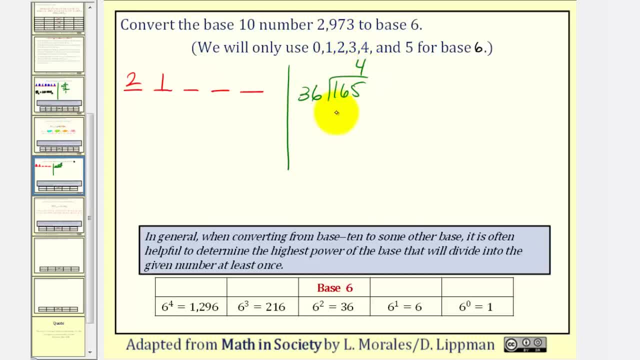 36 goes into 165. four times Four times 36 is 144. The remainder of 21.. So our next digit is four, which will be in the sixth of the second place value. here We'll repeat using 21.. Six divides at least once into 21..